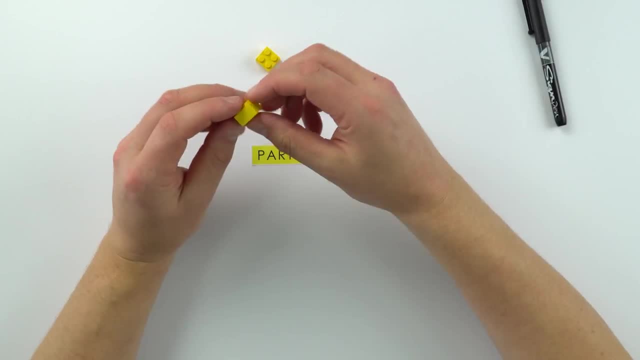 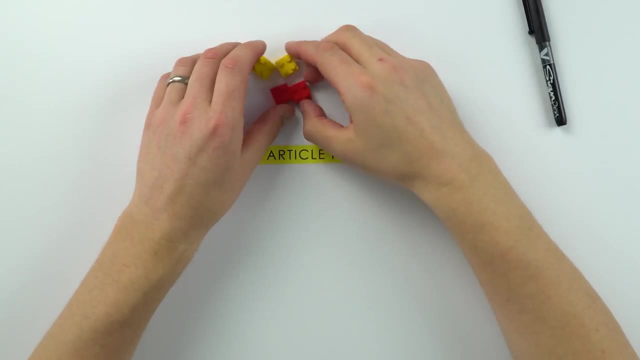 and neutrons And for the purpose of this video and all the others I've done, I'm using just these yellow Lego bits to be my protons. There's no reason, it's just a way to model it. So we've got protons and neutrons, we've got this dense nucleus. 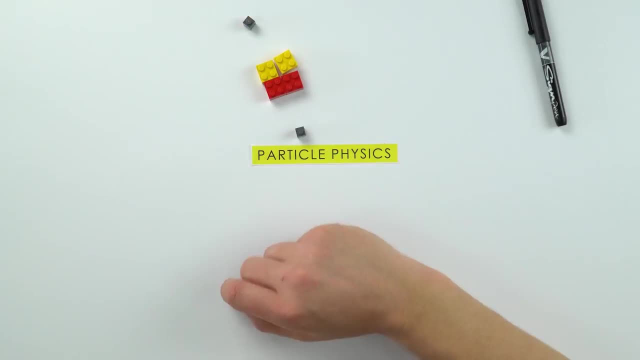 here and surrounding that we have shells of electrons which I'm just using, these one by one grey pieces of Lego. So what do you know from GCSE? So here we've got a proton, we've got a neutron and an electron. Now, at GCSE, we tend to talk about 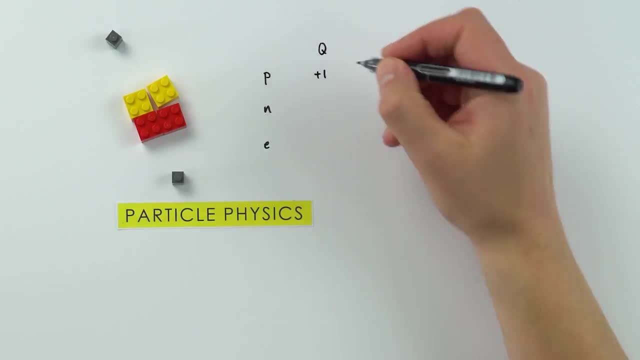 the charges on these of a proton being positive, a neutron zero and an electron is negative. Now, really, these are just the relative charges At A-level. we actually quantify the charge in coulombs and basically a proton has a charge of plus 1.6 times 10 to the minus 19. 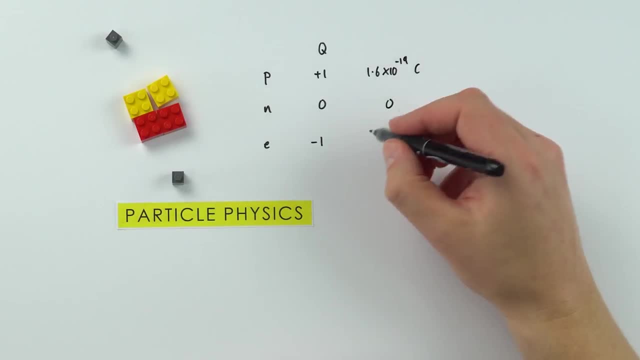 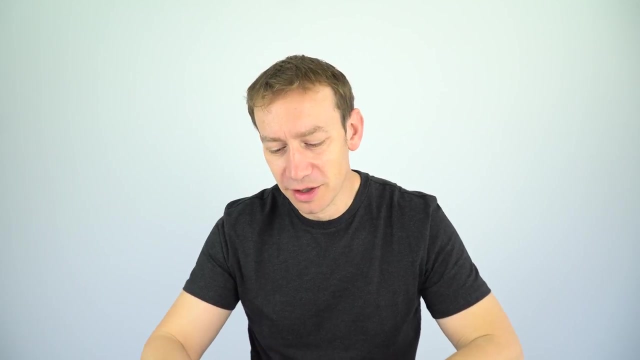 coulombs, a neutron is zero and the electron is minus 1.6 times 10 to the minus 19 coulombs. And what we say is that this value here is the elementary charge. This is the smallest unit of charge that I guess charged particles come in. So 1.6 times 10 to the minus 19 coulombs. 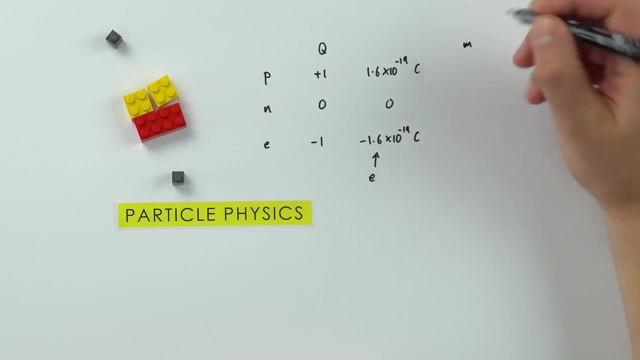 Likewise with the mass. when it comes to looking at the mass of these particles, we tend to say that a proton's got a mass of 1,, a neutron's got a mass of 1, and an electron is maybe two thousandths of that. But again, this is just the relative masses of these things. 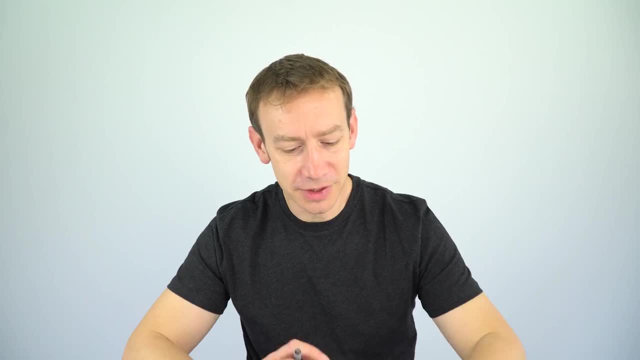 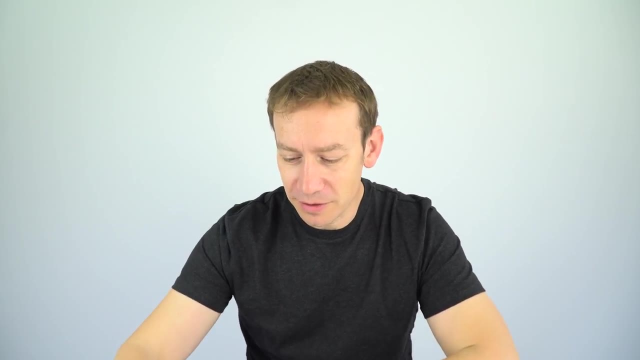 We actually maybe want to quantify this in kilograms. So if we were to take maybe one of these protons and we put it on a very small weighing scale and it wasn't moving, so this is the rest mass- we'd actually find that for a proton. 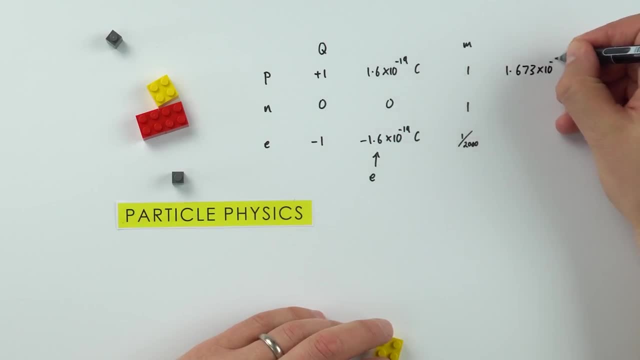 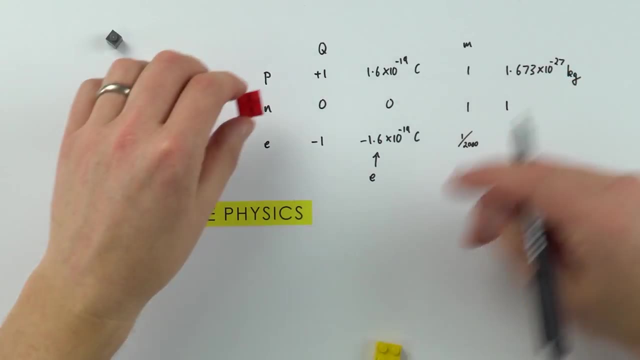 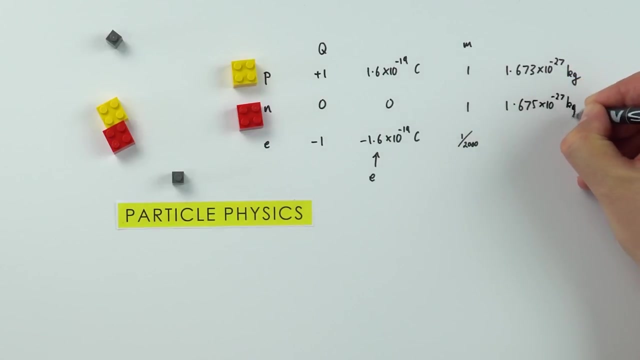 it's equal to 1.673 times 10 to the minus 27 kilograms. Okay, so that's really really light. If we were actually to look at one of these neutrons that we have over here, that's 1.675 times 10 to the minus 27 kilograms and the rest. 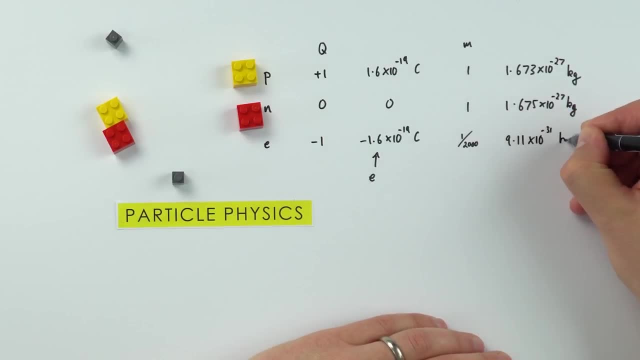 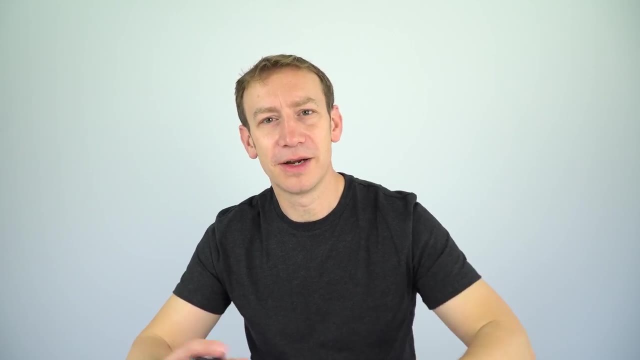 is 9.11 times 10 to the minus 31 kilograms. Okay, so this number here you will be very familiar with. We're often looking at the mass of electrons, especially when they're being accelerated. So that's some stuff that we know from GCSE and how we extend it a bit. 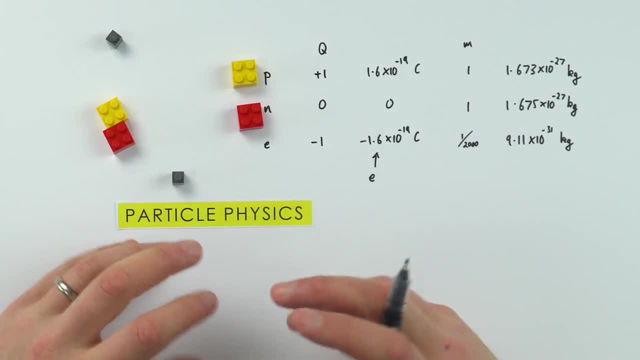 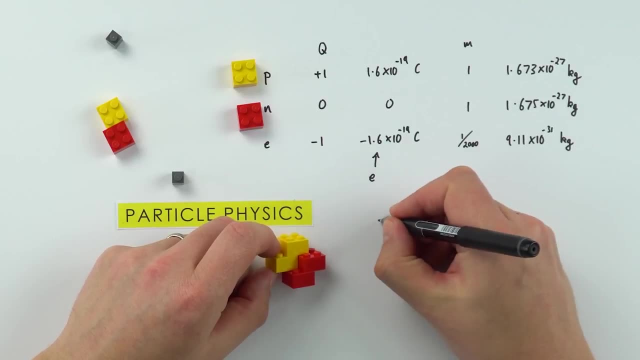 as we go into A level Again. if we have an atom, maybe we've got two protons and two neutrons. we can represent this In this case. this one here is helium and we've got helium-2, protons, and 4 is the total number of bits inside. Now the number at the bottom is Z and the number 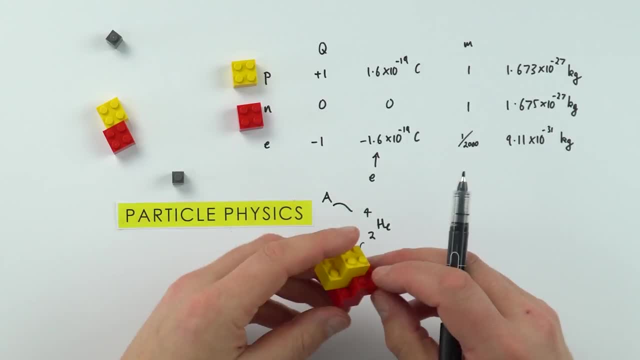 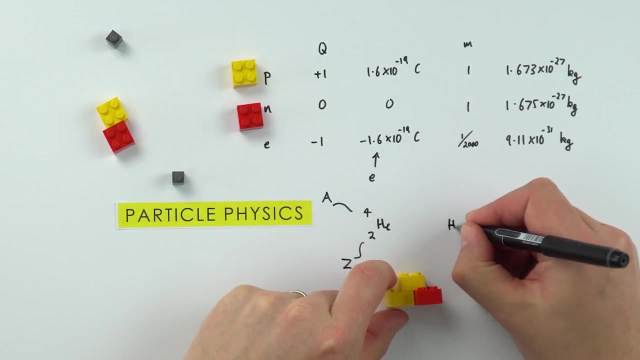 at the top is 8.. We also have some things which might have the same number of protons but a different number of neutrons. This one over here, for example, it's still helium because it still has two protons, but now it's got three things in the middle and this is an isotope. So isotopes. 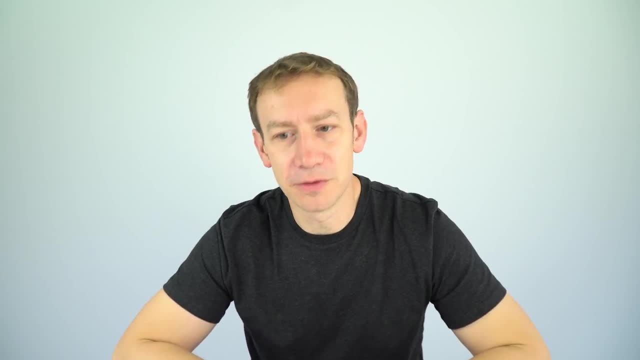 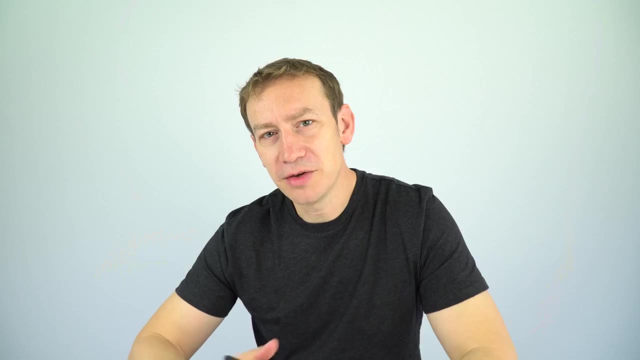 it's just the same element with a different number of neutrons. So, again, that's just what you know about from GCSE. and when it comes to looking at isotopes, what we spend a lot more time- especially as we go through the A-level course- looking at are the unstable isotopes and we call 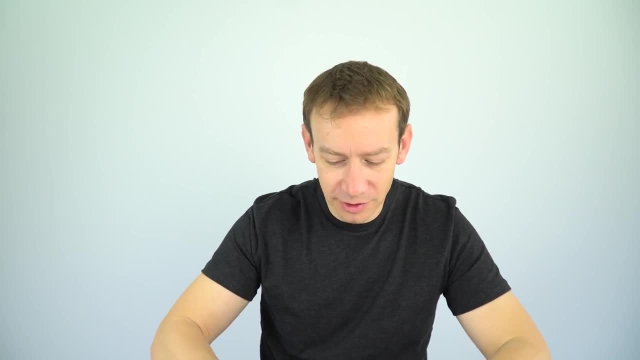 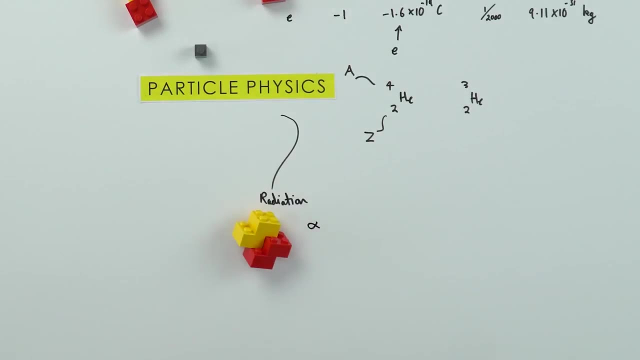 these radioisotopes, and that leads on to things like radiation. So at GCSE we maybe talked about alpha radiation, which is two protons and two neutrons. We also talked about beta, which is basically a high-speed electron ejected from the nucleus. Well, now we go on to different sorts. 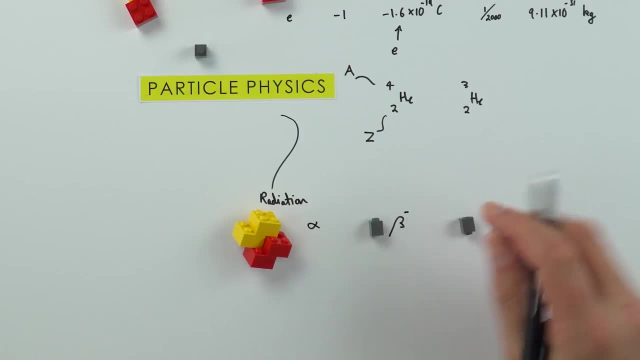 of neutrons and we talk about beta, which is basically a high-speed electron ejected from the nucleus- beta radiation. because this is an electron, it has a negative charge, so we call that beta minus. We also have beta plus and I've just turned this electron the other way around to show that this. 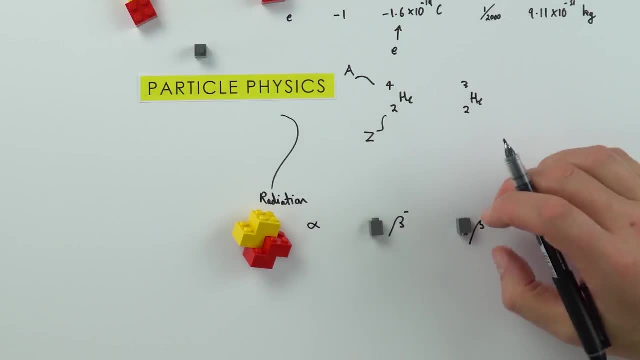 is actually a positron, It's antimatter, and sometimes we have these positive electrons which are emitted from the nucleus, as well as things like gamma, which basically isn't a particle at all. Well, maybe it is because we look at the kind of the particle-like nature of photons later. 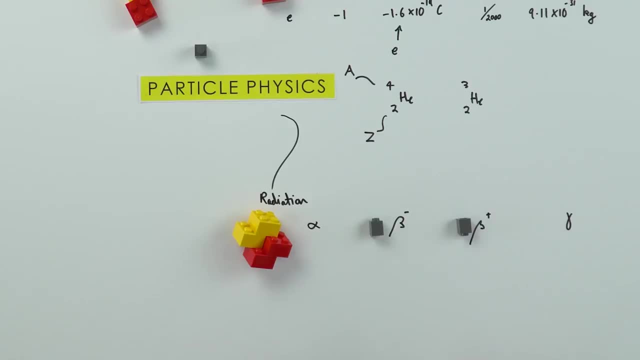 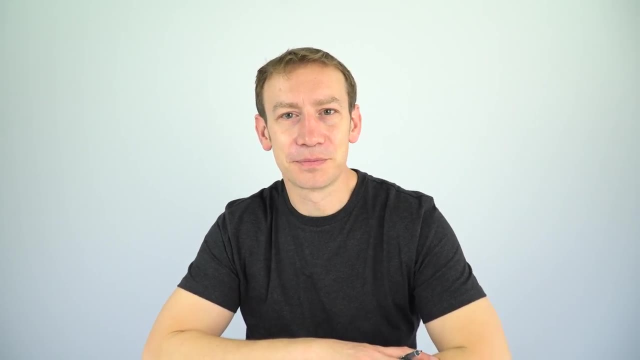 in the course. But yeah, basically this isn't really a particle. It has no mass And, yes, we've got alpha, beta and gamma radiation and as we go through the course we tend to look more at things like half-life. But why is this? 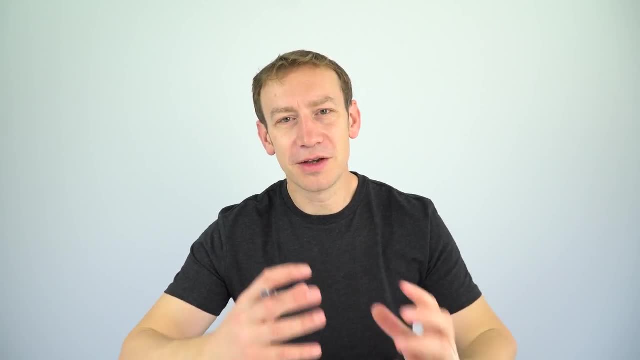 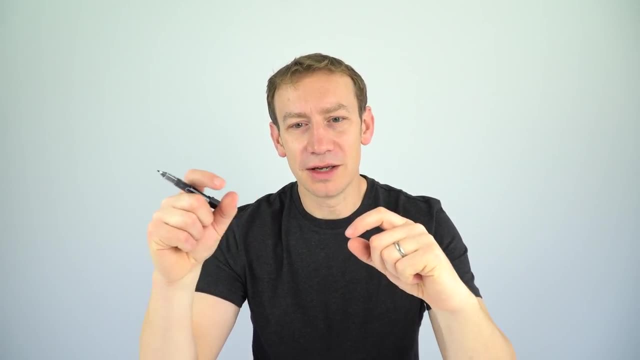 interesting? Well, it's because at GCSE we kind of didn't go into loads of detail. Why is it that we have negative particles which are orbiting a positive nucleus, but yet they don't go straight into it, because there's this attractive force between the two? Why is it that if we have a 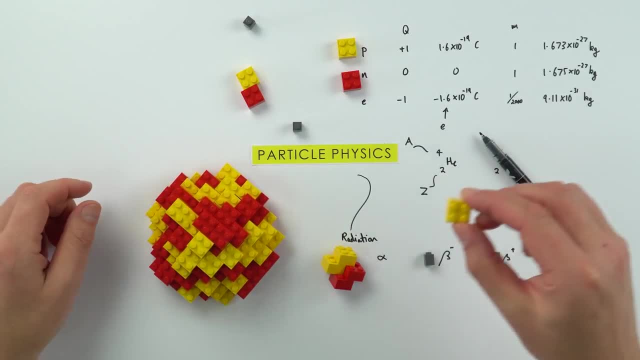 nucleus perhaps like this: and we have a positive nucleus and we have a negative nucleus, and we have a positive nucleus and we have a negative nucleus, and we have a positive nucleus and we have a positive nucleus, and you maybe bring another positive proton towards this big mass of positive things. 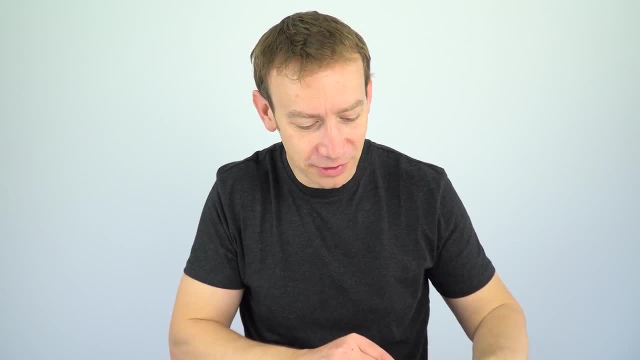 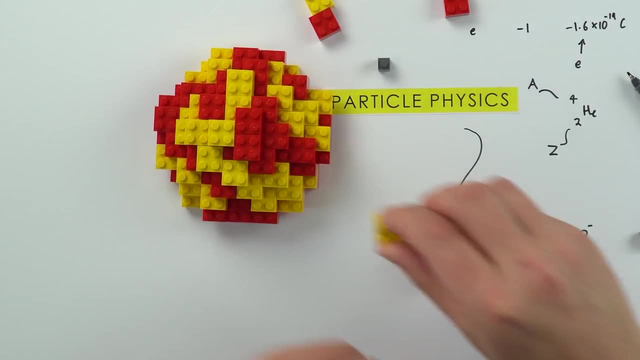 why doesn't it all repel? I mean, we can see this here. As we bring this closer, we can see there's definitely a repulsive force between the two And basically all of these positive protons are pushing away from the other positive protons, spaced apart by some of the neutral. 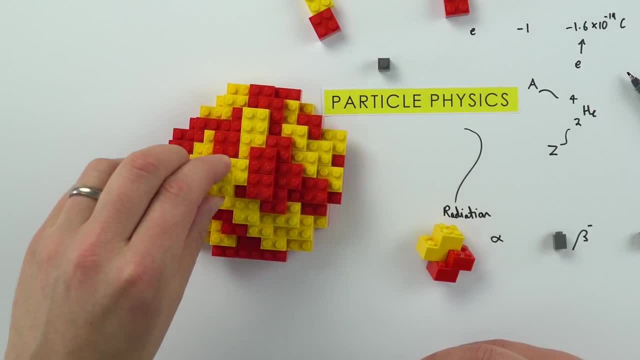 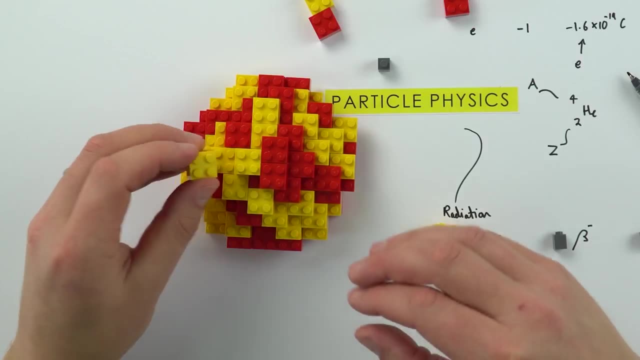 neutrons. But effectively, when this gets really, really close, rather than it being repulsive, suddenly it can actually join on and there's this attractive force. And this is because inside the nucleus we don't just have the normal forces that we're used to, we have this strong nuclear force. 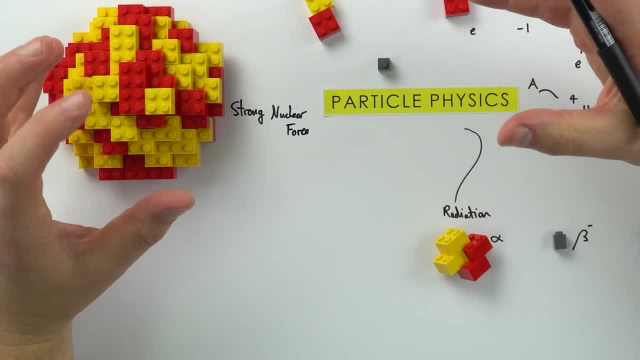 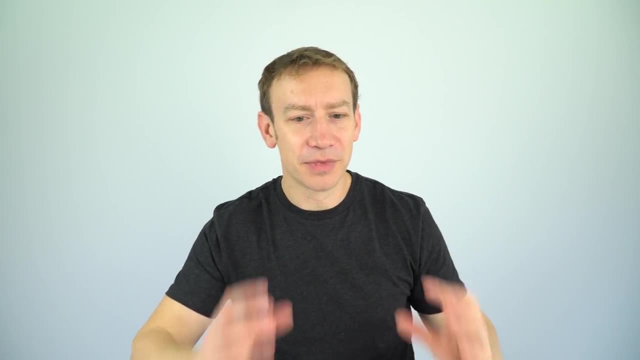 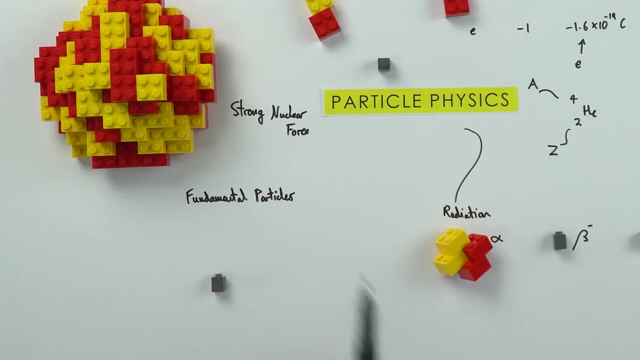 and that overcomes the electrostatic repulsion. And actually, if we start looking more at more detail at these protons and neutrons, we find that we can split them apart. Now this is when we talk about fundamental particles, and the electron is a fundamental particle. We can't split it down. 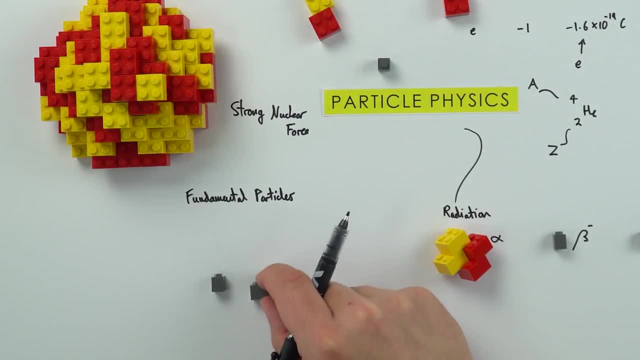 any further. But actually we have things which are like electrons but heavier, and we call these muons. And also we have these really really super heavy electron-like things called Tau particles. OK, so we've got some new particles. we maybe haven't seen that much before Associated with these. 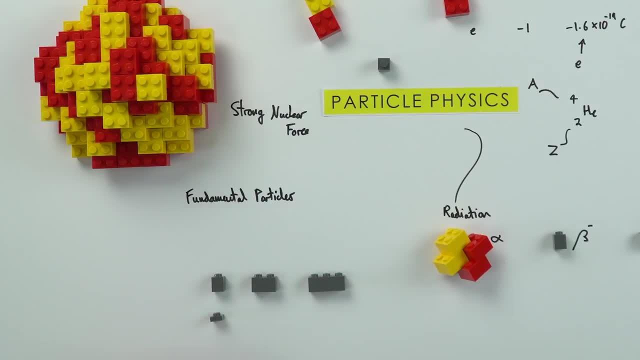 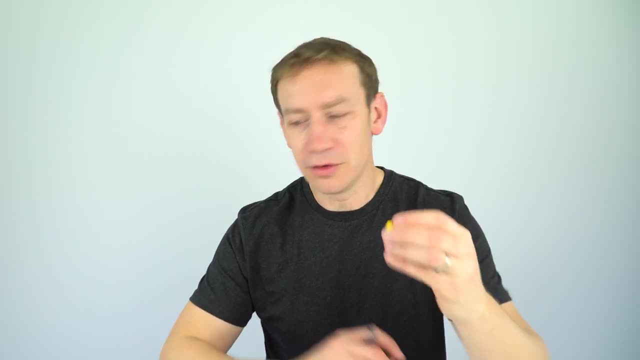 we have neutrinos, So we might have the electron neutrino Again. that was never really discussed. before you get to A level, And if we were to actually split apart a proton or a neutron, we'd find that it's made out of smaller things. 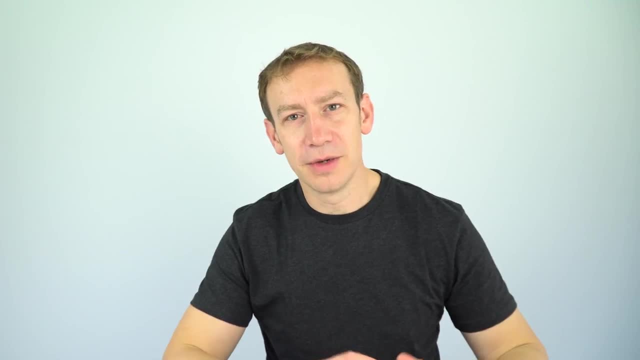 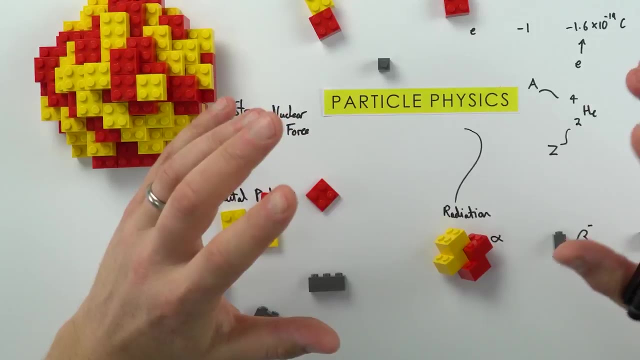 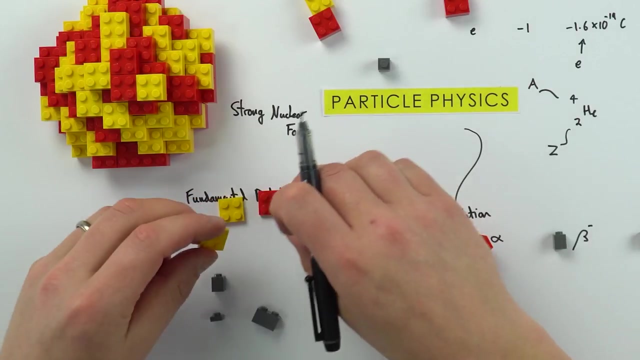 called quarks. Now, quarks can't exist on their own. they come in twos or threes and this is basically a class of particles called hadrons. Now you might be familiar with the LHC. Over at CERN. we have the Large Hadron Collider and hadrons are particles which are made out of quarks. 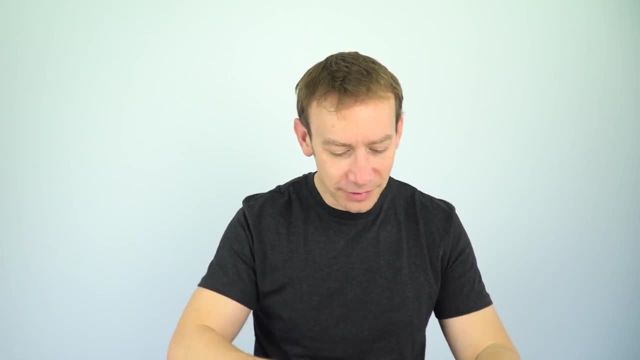 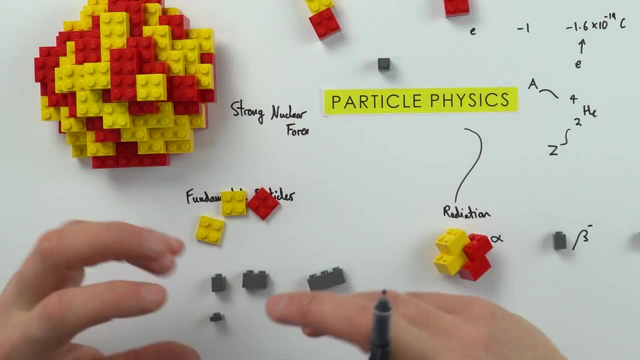 Sometimes they're called quarks. I prefer the name quarks, These ones over here, the electrons and so on. these are actually what we call leptons And basically inside protons and neutrons we have a different combination of quarks. Inside a proton we have two up quarks and a down quark.